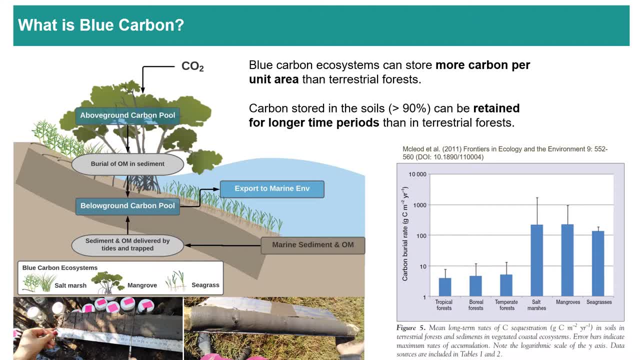 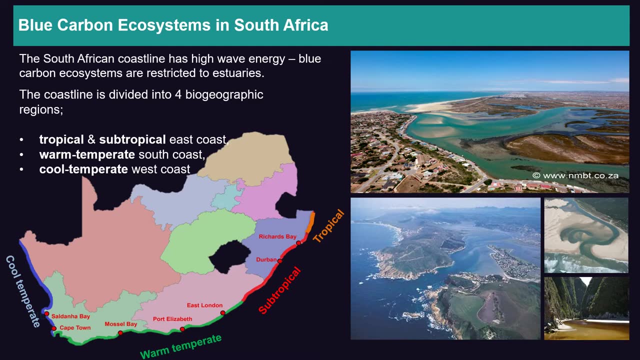 On the lower right-hand side we see the carbon burial rate is higher for mangroves, salt marshes and seagrasses in comparison to terrestrial tropical forests. The South African coastline has high wave energy. This means that blue carbon ecosystems are restricted to occurring in sheltered estuarine areas. 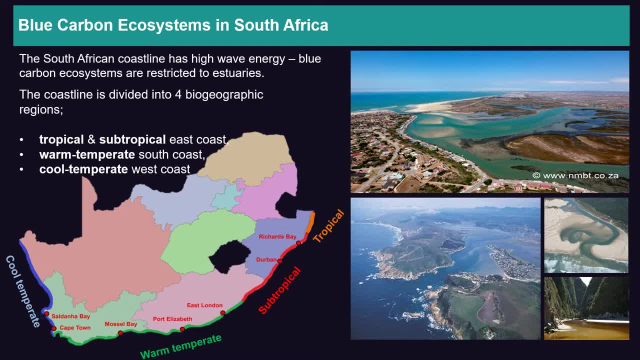 A coast is also divided into four biogeographic regions: The tropical and subtropical ecosystems. The tropical and subtropical ecosystems. The tropical and subtropical ecosystems. The warm temperate south coast. The warm temperate south coast. The cool temperate west coast. 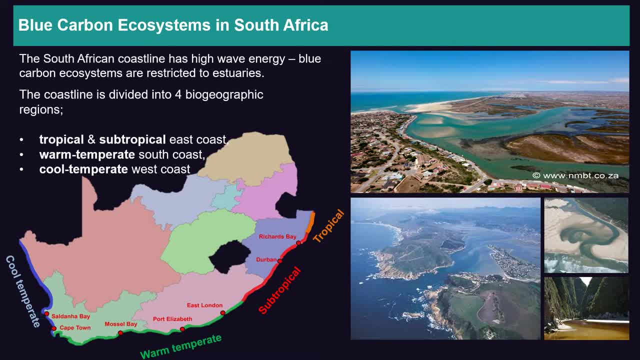 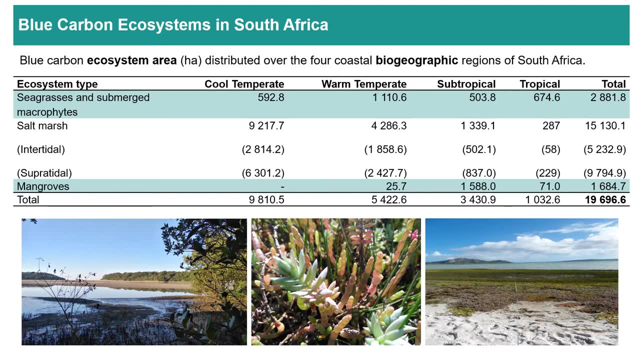 This determines where the different blue carbon ecosystems can occur. Blue carbon ecosystems are distributed over the four biogeographic regions of South Africa. The largest areas are found within the cool temperate bio region. This is because of the contribution of salt marshes. 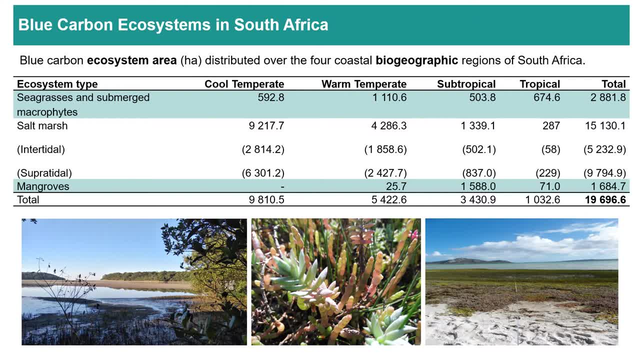 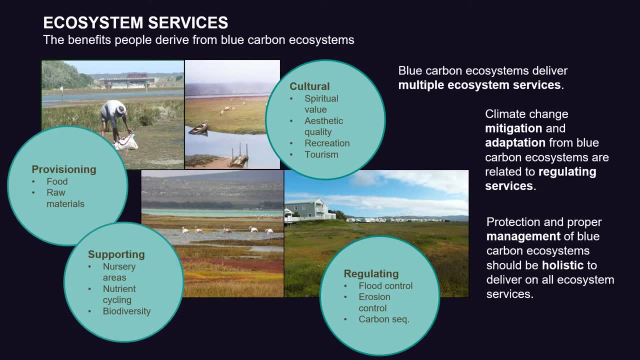 Mangroves occur only from the warm temperate to subtropical and tropical regions. This is because of the contribution of salt marshes. sea grasses and submerged macrophytes cover much smaller area. There's approximately 20,000 hectares of blue carbon ecosystems found in South Africa. Blue carbon ecosystems provide many ecosystem. 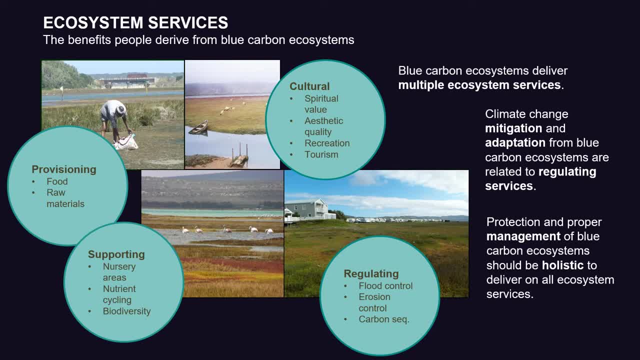 services, and these are the benefits that people derive from these ecosystems. Ecosystem services can be in the form of provisioning, supporting, cultural or regulating services. Climate change mitigation and adaptation from blue carbon ecosystems are related to regulating services. It's important to remember that protection and management of blue carbon ecosystems 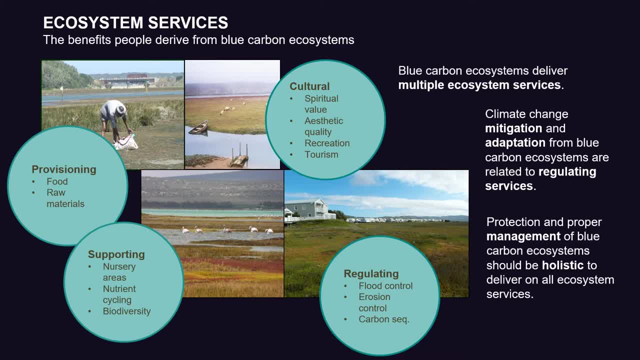 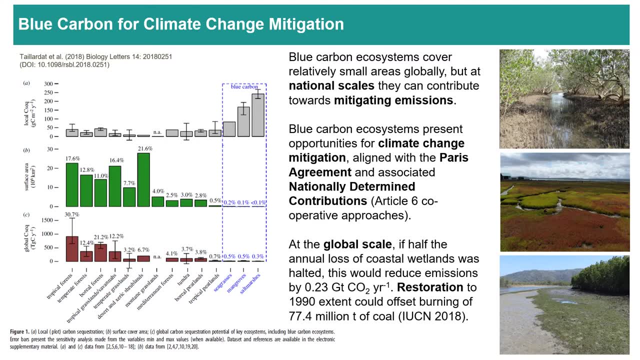 should be holistic so that it can deliver on all ecosystem services. How do blue carbon ecosystems contribute towards climate change mitigation? These ecosystems cover a relatively small area globally, but at national scales they can contribute towards mitigation. Blue carbon ecosystems therefore present opportunities for climate change mitigation. 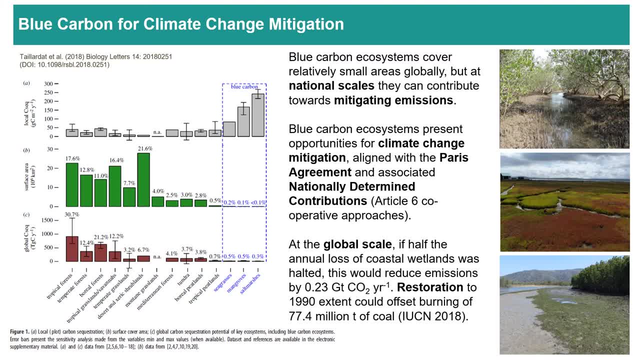 aligned with the Paris Agreement and nationally determined contributions At the global scale. if half the annual loss of coastal wetlands was halted, this would reduce emissions by 0.23 gigatons of carbon Restoration to the 1990 extent could offset the burning of 77.4 million tons of coal. 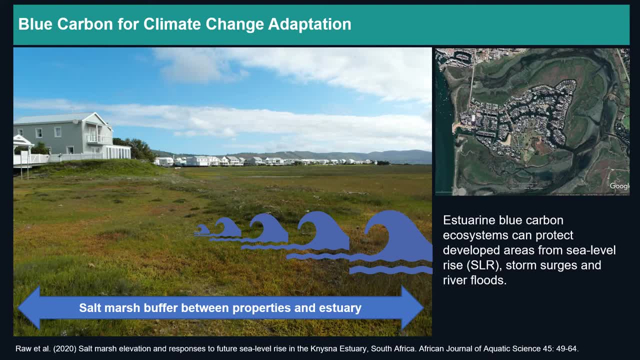 Blue carbon ecosystems deliver on climate change adaptation directly by protecting developed areas from sea level rise, storm surges and river floods. In this example, we see the salt marsh acting as a buffer between properties and the estuary at Nasna. What do we know about blue carbon in South Africa? 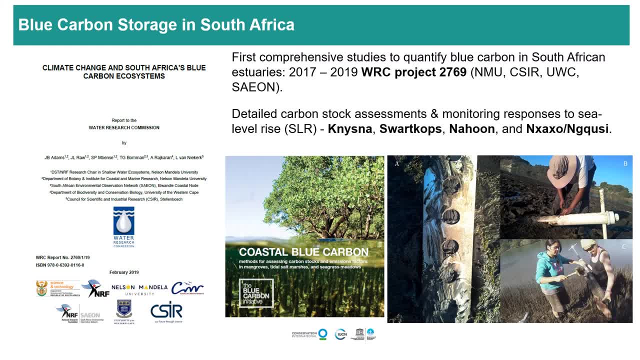 The first comprehensive studies to quantify blue carbon in South African estuaries were carried out between 2017 and 2019 as part of a WRC funded project. Detailed carbon stock assessments and monitoring the responses to sea level rise were measured at the Nasna, Swartkops, Nahoon and Plainhill estuaries. 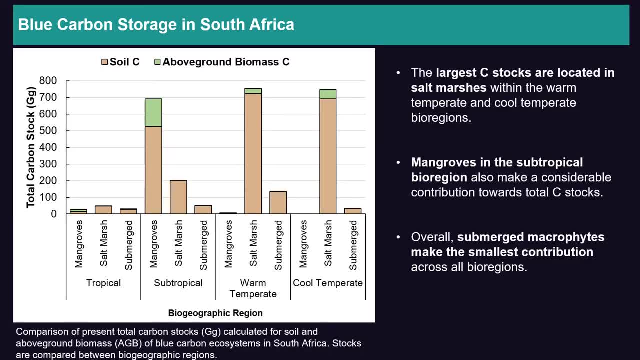 Following on from this study, we were able to extrapolate blue carbon storage nationally. The largest carbon stocks are located within salt marshes of the warm-tempered and cool-tempered bioregions, and this is because this ecosystem is the most extensive. 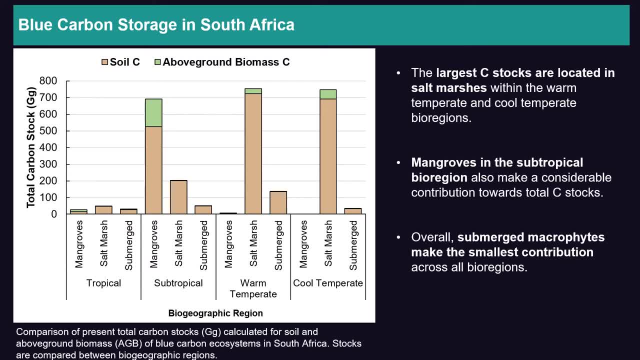 Mangroves in the subtropical bioregion also make a considerable contribution towards carbon stock, and this is because mangroves can store more carbon per unit area in comparison to the high-temperature bioregions, serving as a pre-season source for water storage. and. 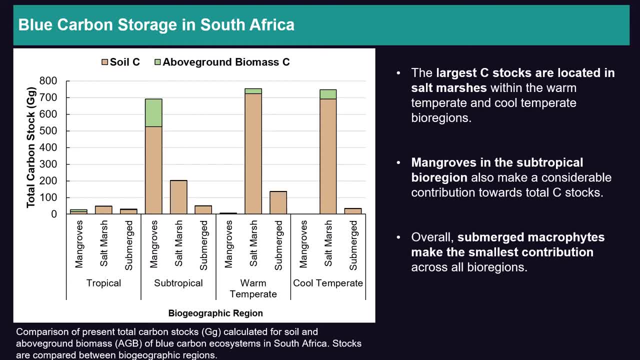 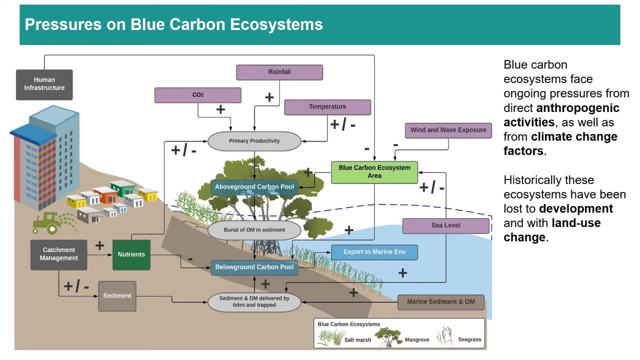 to salt marshes and submerged macrophytes. Overall, the submerged macrophytes make the smallest contribution across all bioregions, Despite the importance of blue carbon ecosystems. they face a number of pressures. These pressures are from direct anthropogenic activities indicated. 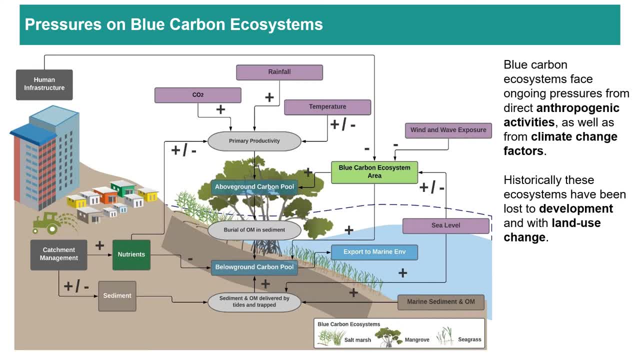 here in the grey, as well as from climate change factors indicated here in the purple. As these ecosystems occur within the coastal zone, they have historically been lost due to development and land use change. Degradation and destruction of blue carbon ecosystems releases the stored. 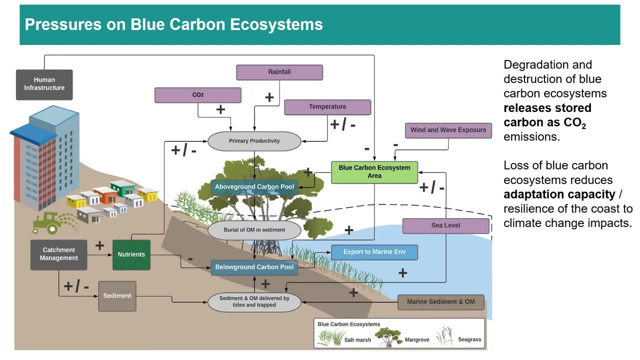 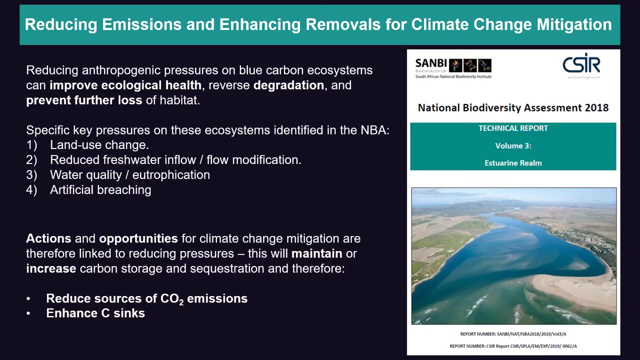 carbon as CO2 emissions. Therefore, losing blue carbon ecosystems reduces the adaptation capacity and resilience of the coast to respond to climate change impacts. Reducing anthropogenic pressures on blue carbon ecosystems can improve ecological health, reverse degradation and prevent further loss of habitat. There were specific key pressures: 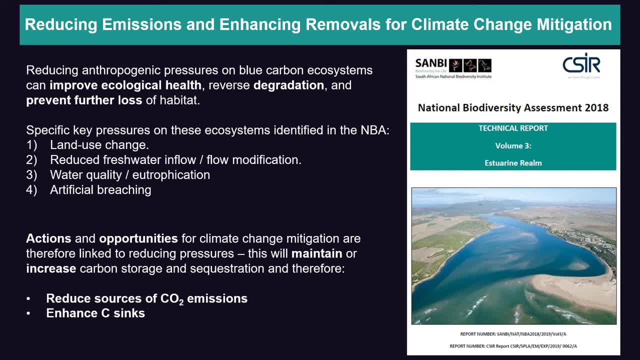 for these ecosystems that were identified in the 2018 National Biodiversity Assessment. These include land use change, reduced freshwater inflow or flow modification, reduced water quality or wetlands flow and reduced drinking water quality. Actions and opportunities for climate change. 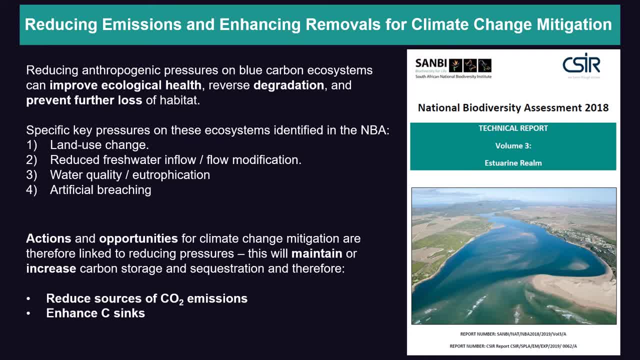 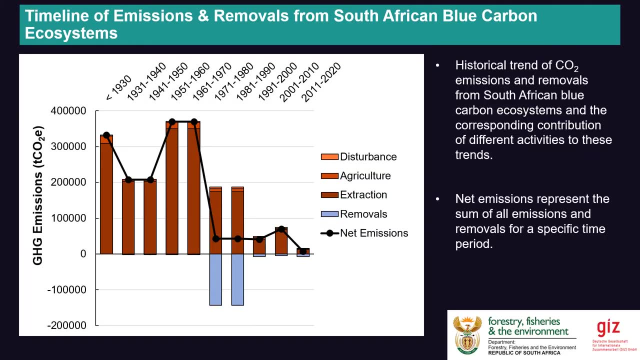 mitigation are therefore linked to reducing these pressures, as this will maintain or increase carbon storage and sequestration and therefore reduce sources of emissions occurring from habitat loss and enhancing carbon sinks. Considering the trajectory of emissions and removals from South African blue carbon systems, we can see the historical trend of emissions and removals. Thus, due to the time of the global warming and the climate change, chlorination and lateral growth, we can see some preserve and reduce the amount of carbon per acre. Using these as the HRDs sources, we can then increase the coast, the pace and climate change mitigation. These can include the use of carbon storage for the environment and to reduce major environmental environmental impact. 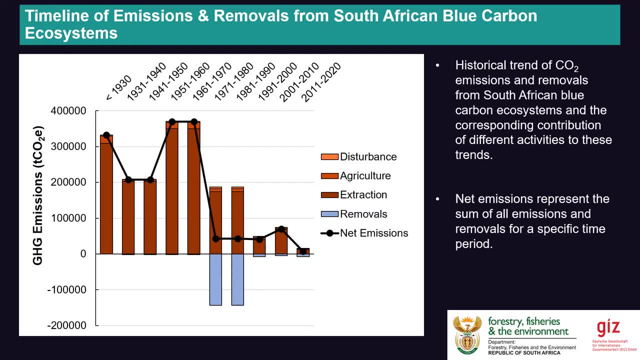 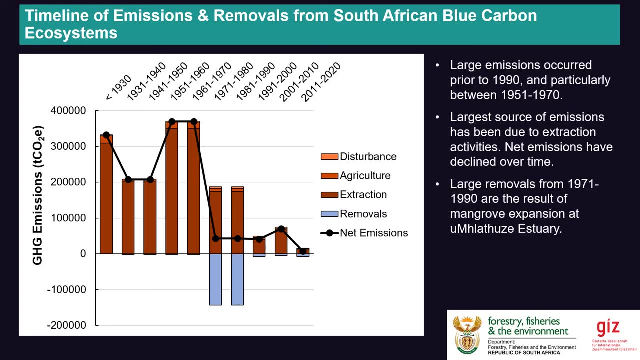 removals over time. The net emissions represent the sum of all emissions and removals for a specific time period. Here we also see the contribution of different activities to those trends. The largest emissions have occurred prior to 1990 and particularly between 1951 to 1970. 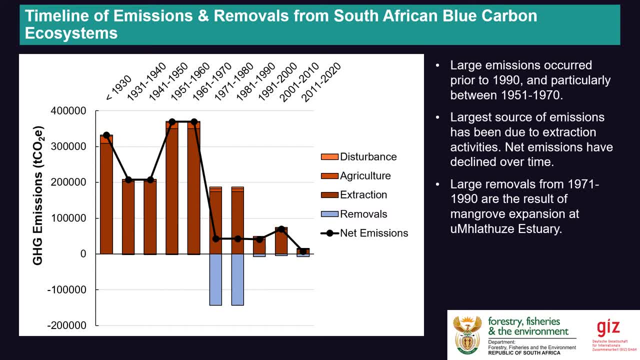 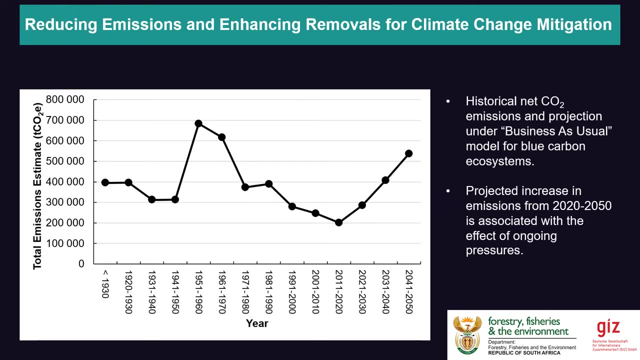 The largest source of emissions has been due to extraction activities, where these represent occasions where bicarbon ecosystems were completely removed and replaced with hard developments or infrastructure. The large removals between 1971 and 1990 are the result of mangrove expansion at Mshletu's estuary. If we consider the historical emissions and removals, 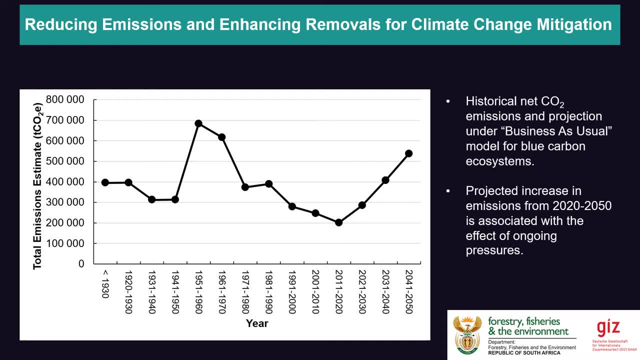 and then project what is expected under a business as usual model, we see that there is an increase in the amount of emissions that are produced in the past year. There is an increase in emissions projected from 2020 to 2050, and this is associated with the effect. 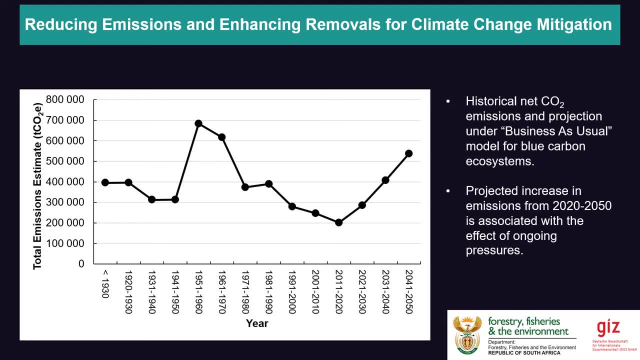 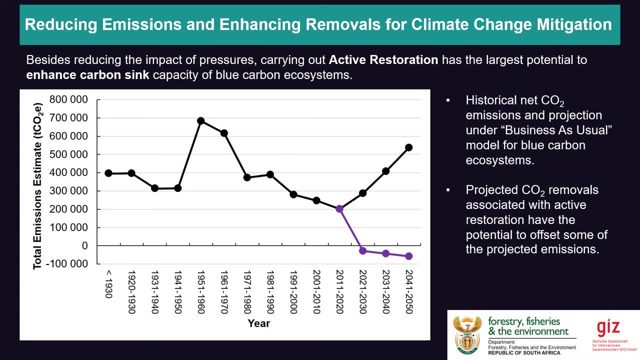 of ongoing pressures on these ecosystems. Besides the impact of reducing these pressures, it is also possible to carry out active restoration to enhance the carbon sink capacity of blue carbon ecosystems. The projected removals associated with active restoration have the potential to increase the carbon sink capacity of blue carbon ecosystems. 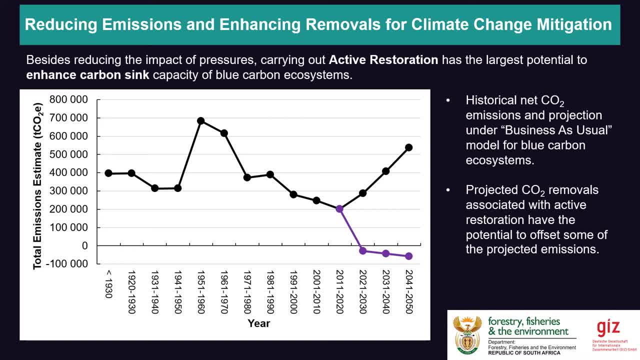 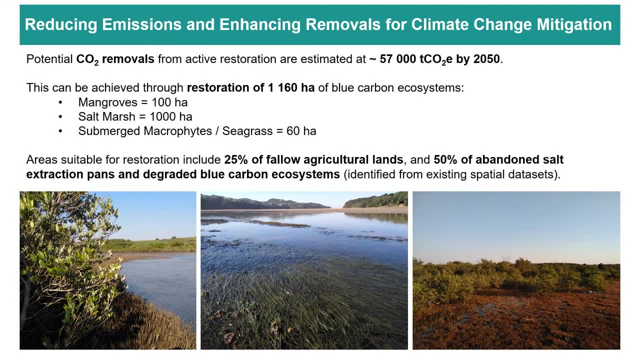 There is also a potential to offset some of these projected emissions going forward from 2020 to 2050.. In summary, the potential CO2 removals from active restoration are estimated at approximately 57,000 tons of carbon dioxide equivalent by 2050. And this can be achieved through the restoration. 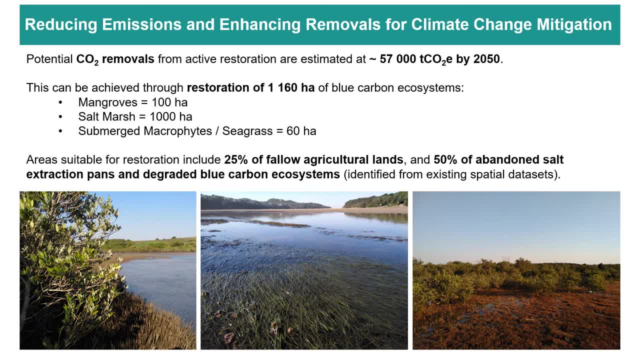 of the life of 1,160 hectares of blue carbon ecosystems, With a considerable adjustment to the, with a contribution of 100 hectares of mangrove, 1,000 hectares of salt marsh and 60 hectares of submerged macrophytes or seagrasses. 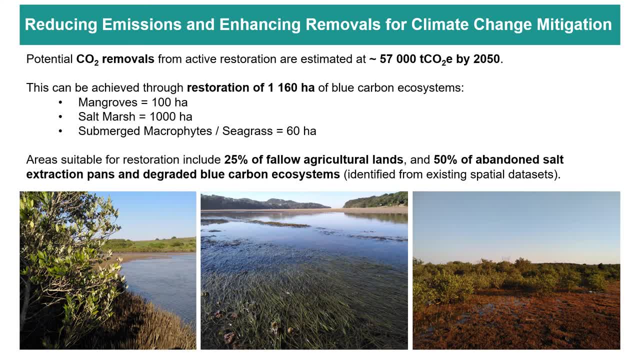 These areas that are suitable for restoration include 25% of fallow agricultural lands and 50% of abandoned salt extraction pans and degraded blue carbon ecosystems, And these have been identified from existing spatial data sets, so these targets are expected to be realistic but conservative. 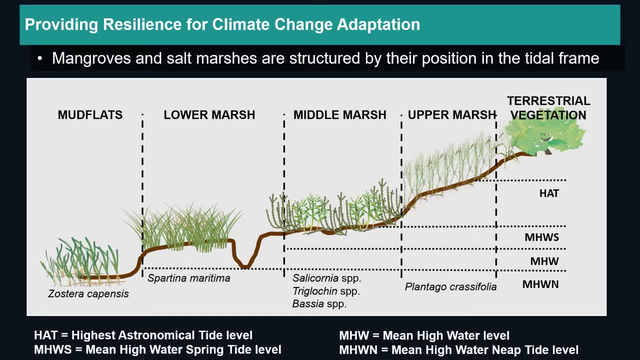 If we consider, next, the potential for blue carbon ecosystems to provide resilience to climate change adaptation, we must first recall that mangroves and salt marshes are structured by their position in the tidal frame, where different plant species occur within different zones, depending on the amount of inundation that they can withstand. 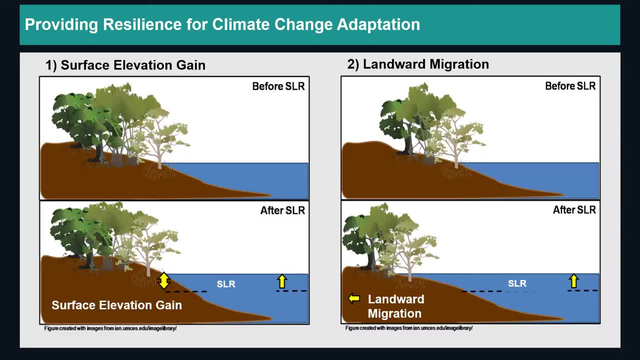 There are therefore two responses, The first one being surface elevation gain, where the ecosystem accumulates sediment and organic matter at a rate that is equal to sea level rise. In this way, the vegetation can maintain its optimal position within the tidal frame. The other alternative is landward migration, whereas with sea level rise, the ecosystem successively moves landward. 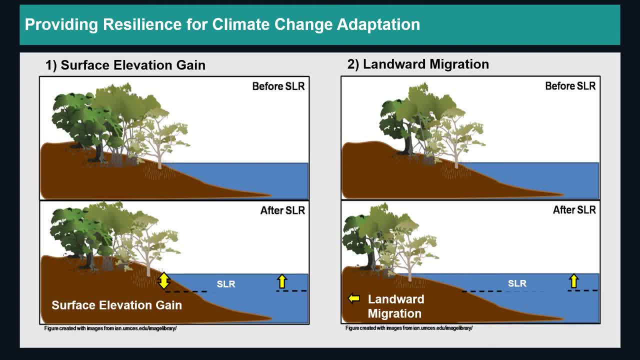 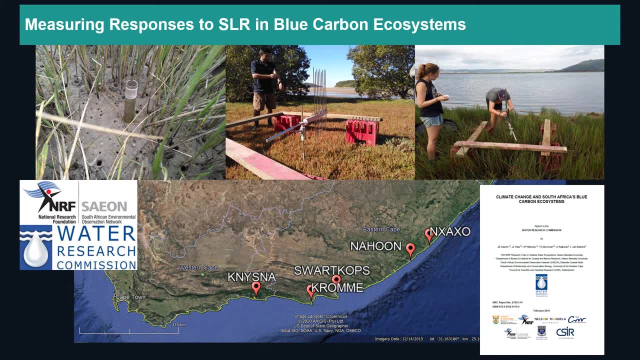 in the form of a sea level rise. The other alternative is landward migration, whereas with sea level rise, the ecosystem successively moves landward in order to maintain a suitable position within the tidal frame. We have been measuring these responses to sea level rise in blue carbon ecosystems of South Africa. 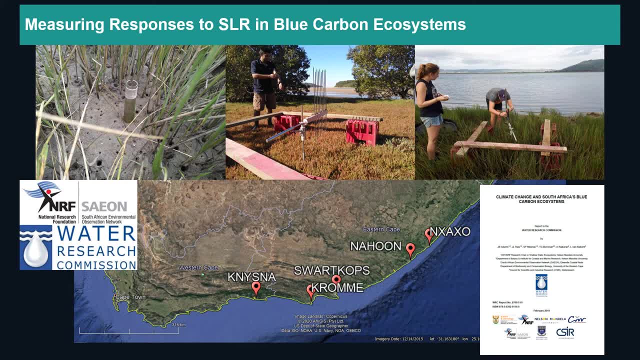 and this was carried out as part of the same WRC project and in collaboration with SEON. There are currently five monitoring sites for blue carbon ecosystem responses to sea level rise, and these are at the Knysna, Crum, Swartkops, Nahoon and Glanmel estuaries. 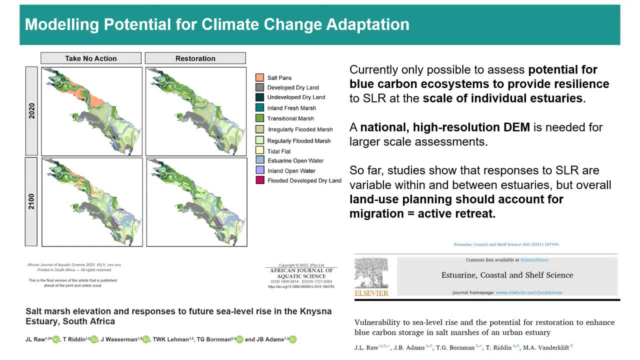 The next step is to go from measuring responses to modeling the potential for these ecosystems to contribute towards climate change adaptation. Currently, this is only possible to carry out at the scale of individual estuaries, and this is because a national high-resolution digital elevation model is needed for larger scale assessments. 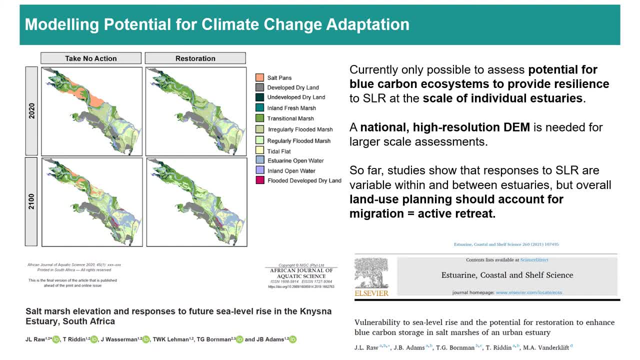 So far, studies that show the responses of sea level rise are variable, both within and between estuaries. However, overall there is going to be a need for land use planning to account for migration and to promote active retreat of developed areas. 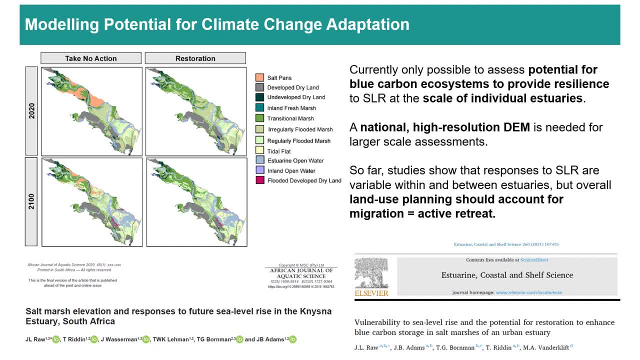 This is because, in most cases, the surface elevation gain rate is not going to be fast enough to cope with sea level rise. The blue carbon ecosystems therefore need space with which they can move back into and therefore continue to provide resilience against sea level rise. 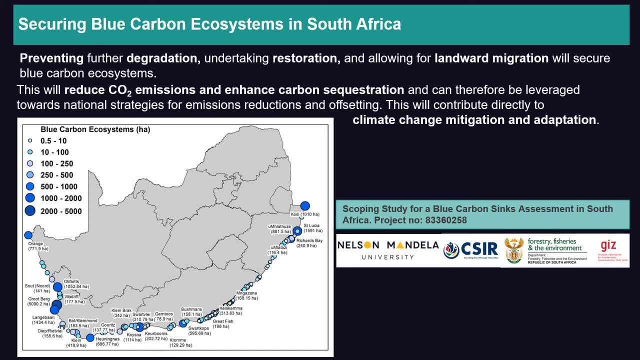 Therefore, preventing the further degradation, undertaking restoration and allowing for landward migration will secure the blue carbon ecosystems in South Africa. This will reduce CO2 emissions and enhance carbon sequestration, and can therefore be leveraged towards national strategies for emissions reductions in South Africa. 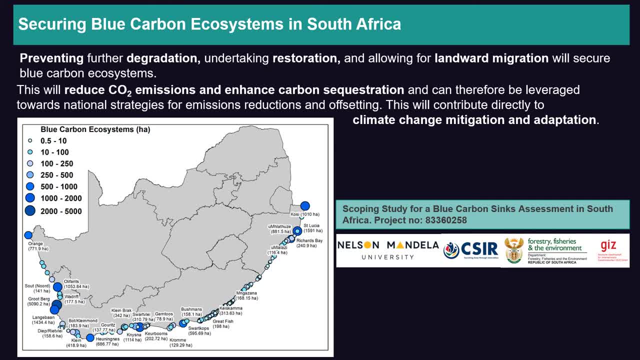 In particular, carbon sequestration is the most level of carbon that you can look at in an ecosystem. We have already done some research on how to address climate change mitigation and offsetting, and this will contribute directly towards climate change mitigation adaptation. This research is currently being carried out as part of a project with the Department of Forestry, Fisheries and the Environment, funded by the GIZ. 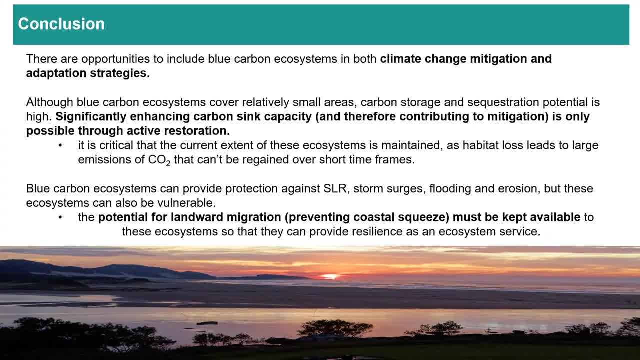 In conclusion, there are opportunities to include blue carbon ecosystems in both climate change mitigation and adaptation strategies, Although blue carbon ecosystems are indeed the most efficient and most lucrative energy platforms, but they also have many potential challenges. So, in particular, we are continuing to do our work, in effect, in the context of the commitment that we have made to climate change mitigation.